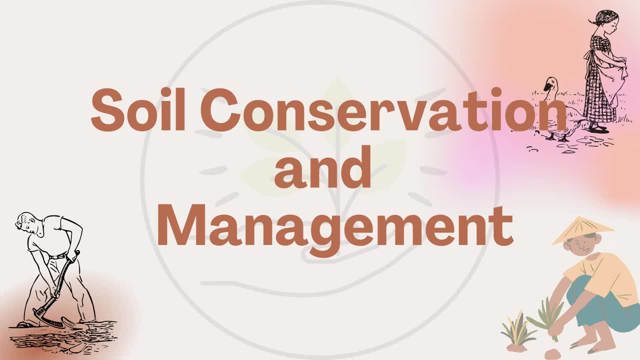 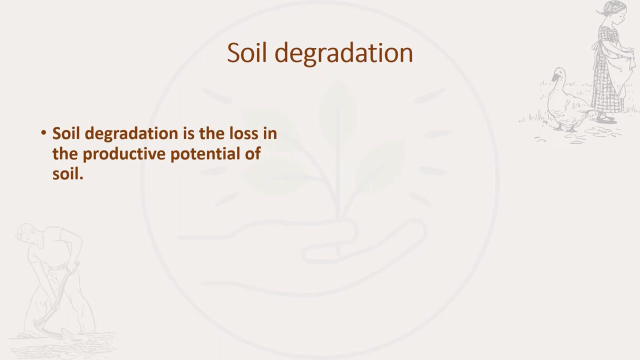 Greetings and welcome everyone. Today, we'll be discussing soil conservation as well as management. We'll be discussing the concept of soil degradation, the types of soil degradation, as well as the impact of soil degradation on agricultural productivity. Now you will recall that on our previous lesson on resources, we mentioned that soil is a non-renewable resource, and why is that so? 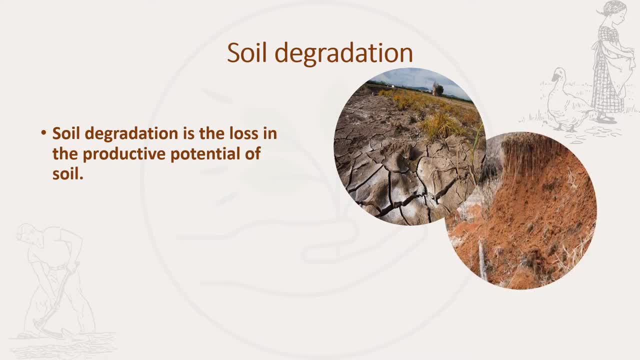 Why is that so? It's because that soil is a mixture of organic as well as inorganic matter and it takes like thousands of years to form. So it may happen sometimes that the condition of the soil changes, Changes and also the soil loses its nutrients, and we call this process soil degradation. 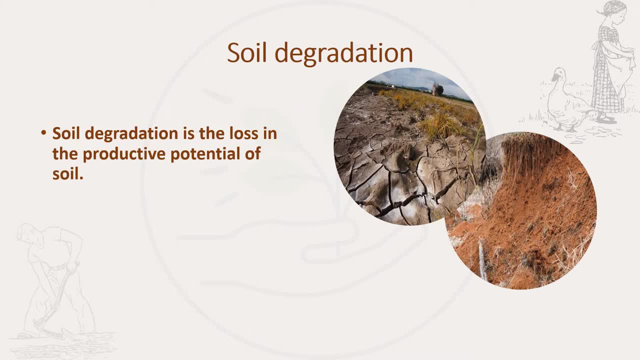 Therefore, soil degradation is the loss in the productive potential of the soil and this sometimes can be a result of like human activities. And this is a widespread problem in South Africa because it threatens food availability And also agricultural activities. It threatens the agricultural productivity at large. 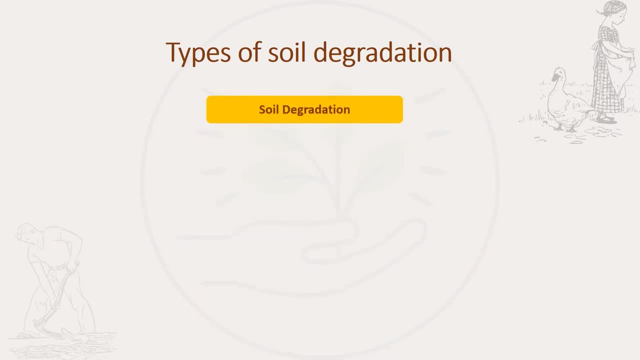 So there are three types of soil degradation and I want us to discuss these three, as these may lead to the loss of soil, And also agricultural activity And emissions. We are talking about crops with fossil fuels, which include raw materials and directly applied to nitrogen-rich soil. 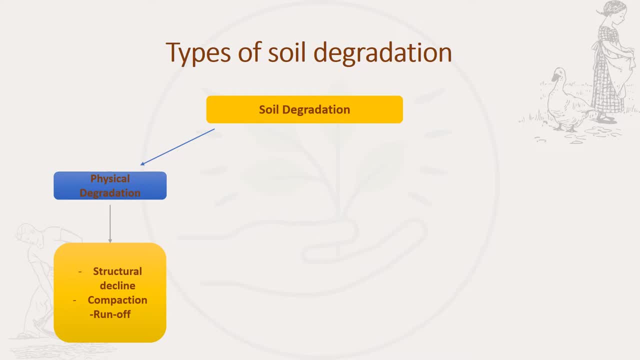 That's right, And it's key factor for soil degradation. We are talking about the ecological species, animals, which may travel over with soil. then the second one, and that i want us to discuss, is chemical degradation. now, with chemical, with chemical degradation, farmers use um a range of 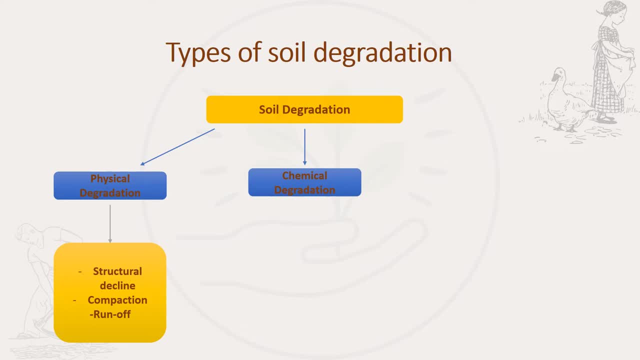 chemicals to kill weeds and pests in the soil. so if these pesticides, as well as habit herbicides, are not applied correctly, the soul may be harmed. now this will lead into acidification, salinization, leaching, nutrient imbalance and also the loss of nutrients in the soil. then the third: 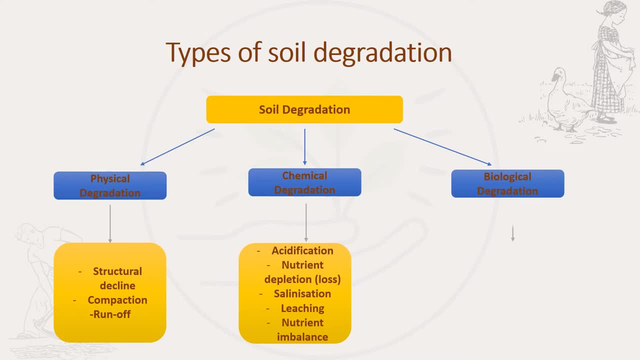 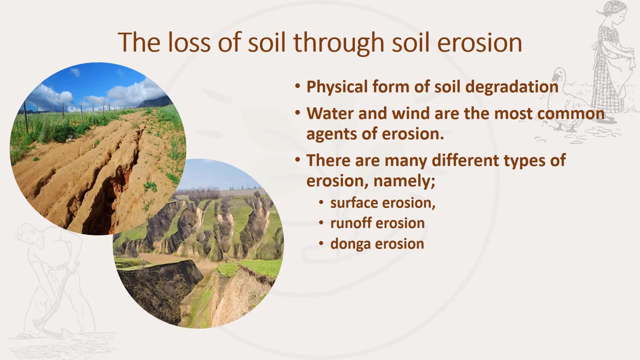 one that i want us to discuss is the biological degradation, and this can lead to the loss of organic um content in the soil. so now i want us to discuss the loss, the loss of soil through soil erosion. so soil erosion, basically, is the physical form of degradation. so when we talk of soil erosion, this is basically the loss of soil itself. 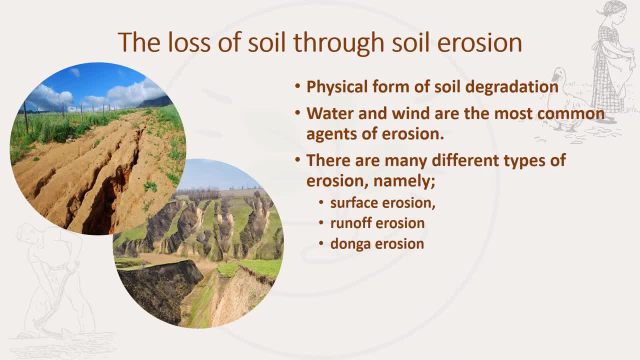 when soil erodes it. الكتنا Tahereω and vou different types of erosion. one of them is surface erosion, and this is where the top layer of the soil is removed, and the other one is a run of erosion. now, this is where a series of 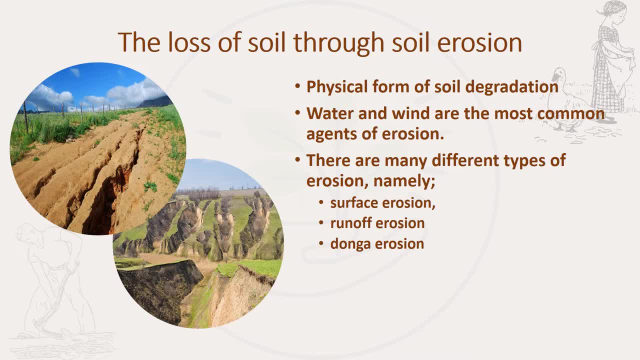 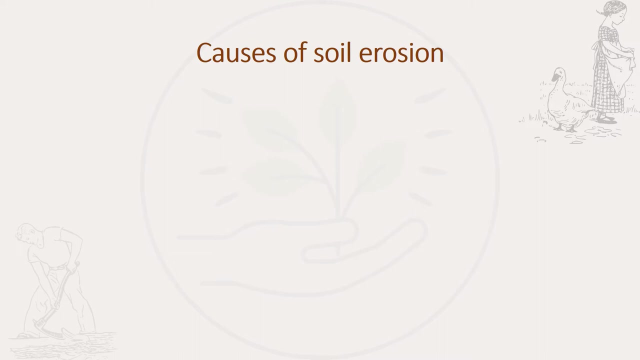 parallel ditches are formed in the topsoil. Then the other one that we have is donga erosion. Now, with donga erosion, there are deep ditches which are formed. So now, what causes soil erosion? So, basically, soil erosion is caused by two factors. One, when the plant cover. 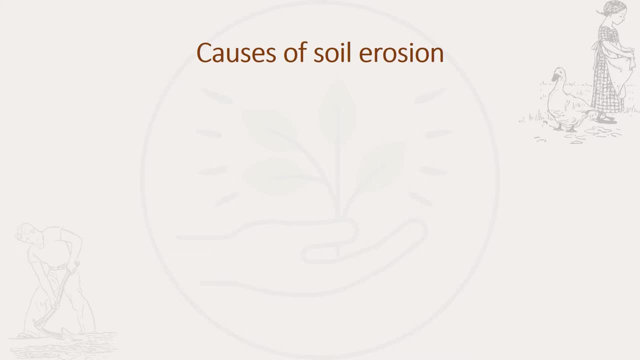 which protects the soil is removed, And secondly, when the slope of the land is too steep. Now, what does this mean? It means that the steeper the land, the greater the rate of erosion. So the causes of erosion may include plowing, overgrazing. 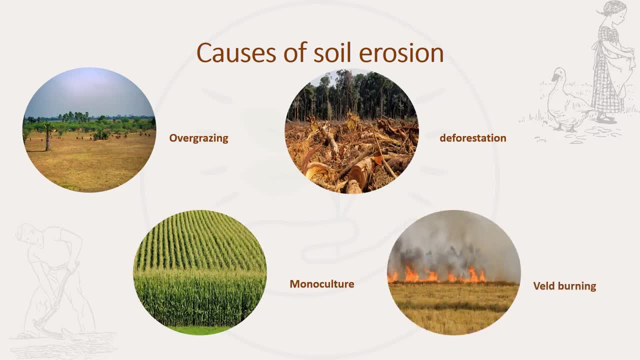 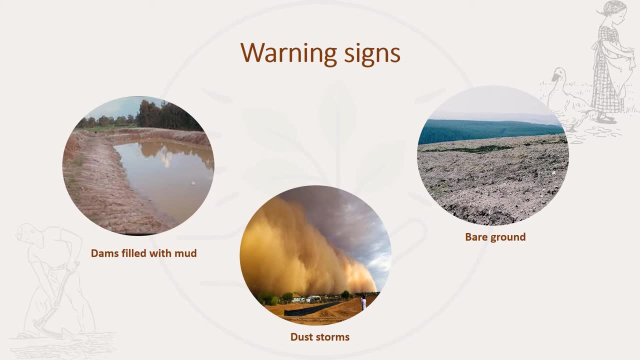 deforestation, monoculture, as well as felt burning. Now that we have talked about the causes of soil erosion, what are the warning signs which one should look for when it comes to soil erosion? What do we look for when we suspect that the soil has been washed away? 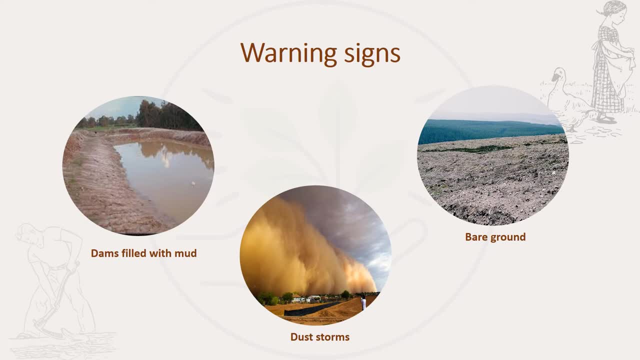 So when there is mud in a dam, This can be a result of soil that has been washed into the dam by flowing water. This is a result of soil erosion, And the other one is that there would be dust storms. So when it's dry, when it's dry and the soil is not held down by plants any strong, 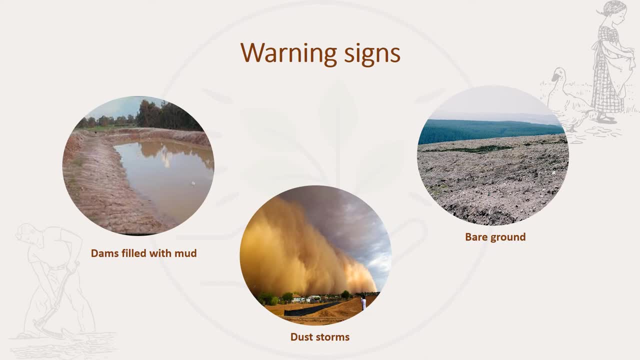 breeze will cause a dust storm, So this too results in the loss of soil, especially with the fertile topsoil. And also another warning sign is the background. Now, with background, this is where plant growth is poor in that area, because the top layer of the soil has been removed by the soil. As you can see, this is where the soil cover is. it is removed Now with background, this is where plant growth is poor in that area because the top layer of the soil has been removed by the soil. 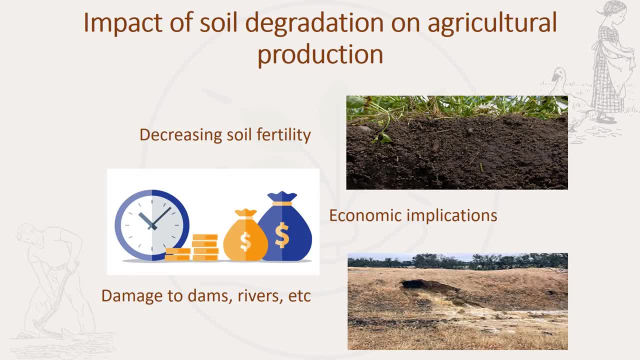 wind. so now I want us to look at the impact of soil degradation on agricultural production, the effects of soil erosion. so soil erosion has three important effects, three effects that we need to consider so that we can try by all means to prevent this type of degradation. so one soil degradation will 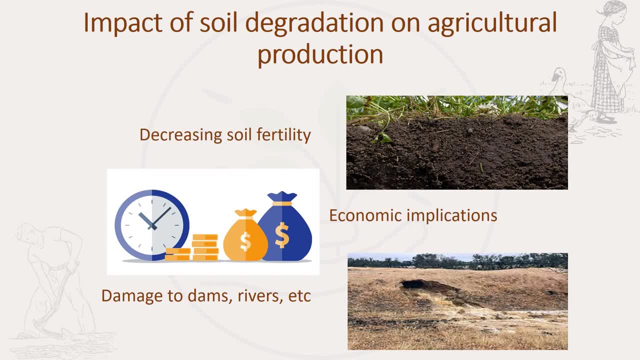 decrease the fertility of the soil. and also, coming to the economic implications- soil degradation makes farming more expensive- and also what it can do. it can increase the fertility of the soil and also the environment. now, this includes the dams of the farm, the rivers and all all the way. now, how do we then control?